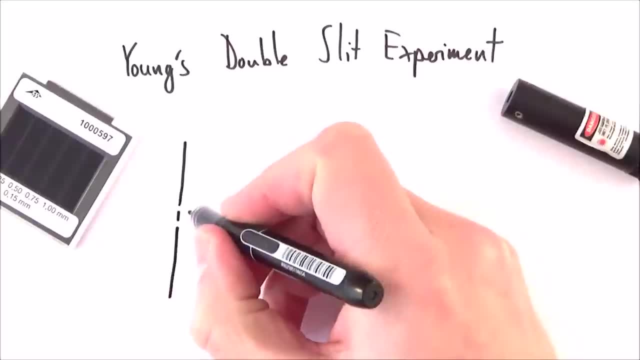 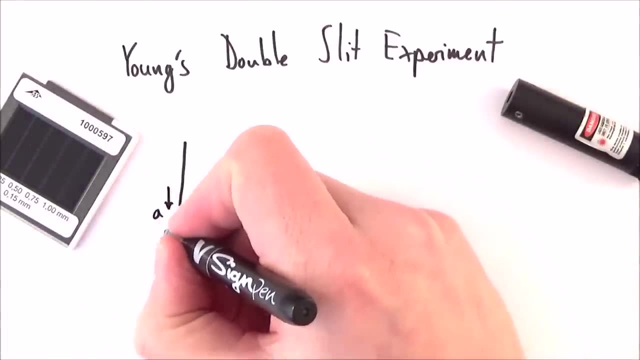 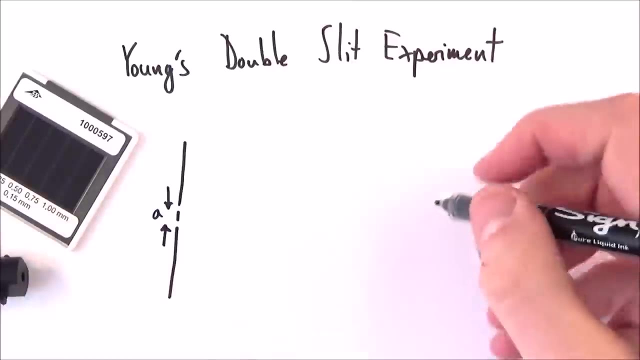 What we have is something with a double slit in it, and we can look at the distance between the two slits as a distance that we call little a. So little a is a slit separation. we then shine the light that's coherent, and we shine it through this onto a screen. Now the 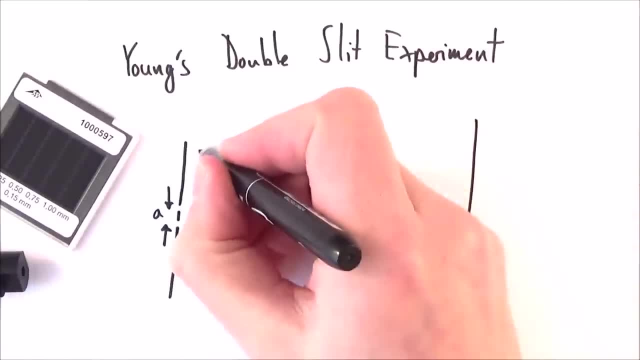 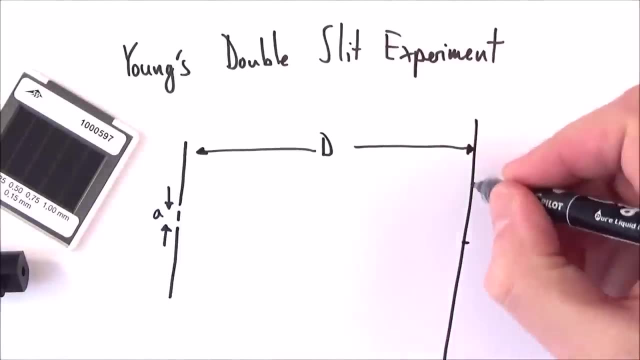 screen is a distance of d meters away. so the distance from the slit to the screen is a distance big d, and what we tend to find is we get a bright point in the middle and then we have a point where there's a destructive interference of light, and then we have another bright point and another. 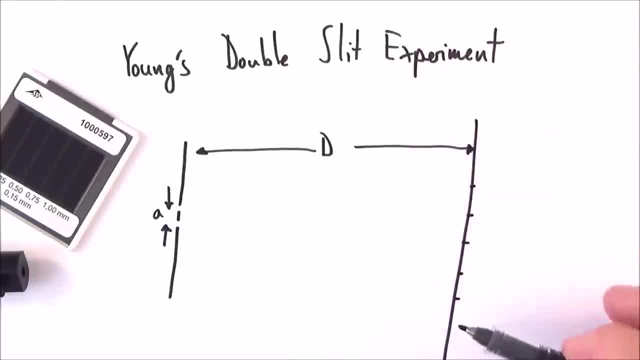 bright point. Now that's not so clear for some good reasons that I'll cover later, but if we sort of have a look at the intensity so we can maybe have a small bright point- gets brighter, we get a massive maximum in the middle, gets brighter and brighter to the sides and it kind of keeps doing. 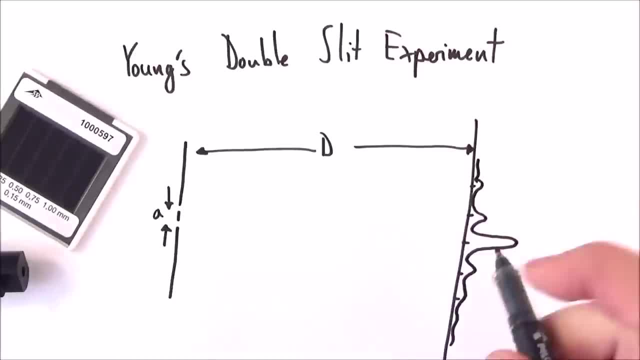 this. What this tends to do is it tends to spread the light out, so we get the brightest point, then it's dark, then it's bright, then it's dark, then it's bright, then it's dark, and what we can look at is the separation of these fringes. Now, in a lab, in the dark, it's a lot easier to measure than 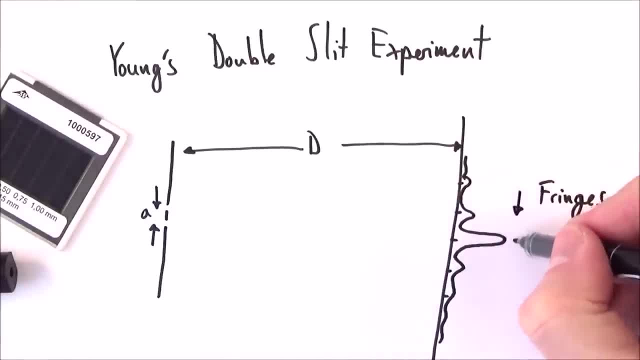 what I've just shown here. but what we can look at is the distance between the two slits, So the distance between fringes as equal to x. and if we look at a, d and x, these are all related to the wavelength of light, and what we find is that the wavelength of light is equal to a x over d, So in 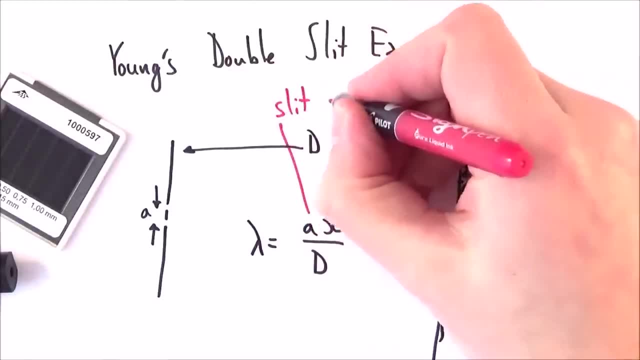 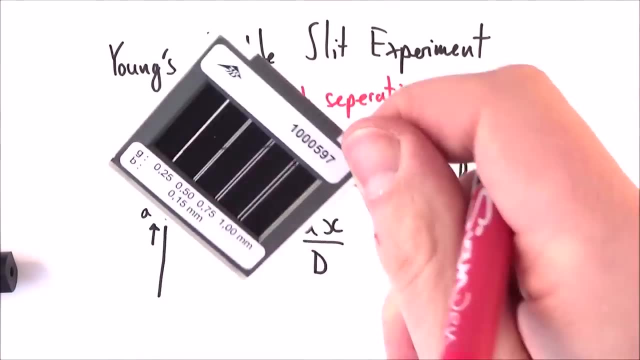 a bit more detail. a is the slit separation, that is, the distance between the slits. Now, often there'll be some information printed on the the thing that you're using, but you can measure it using a traveling microscope. So this is a microscope that moves between the two slits. So this is a microscope that moves between the two slits. 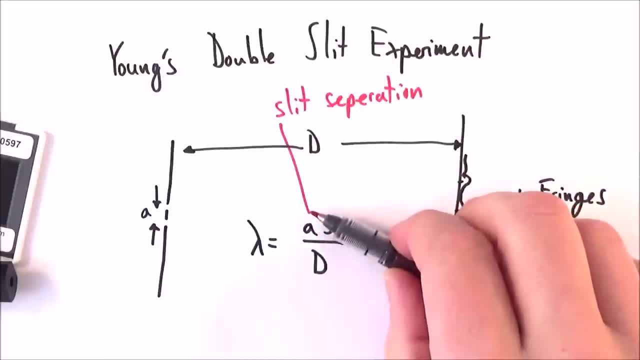 So on a very small distance you can very accurately read the distance or the length of very small objects. X is the fringe separation and we talk about the light and the dark fringes, and it's often easier to measure perhaps a distance of 10 fringes and then divide by 10 to get the distance. 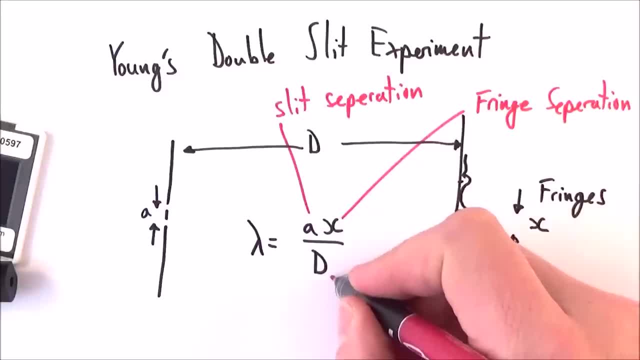 of one, because it's going to be, you know, fractions of a millimeter. And then, finally, distance from whatever you're projecting the light onto from the, the actual slit. that's fairly easy to measure using a meter ruler, You know you can measure the distance between the two slits and then you can.